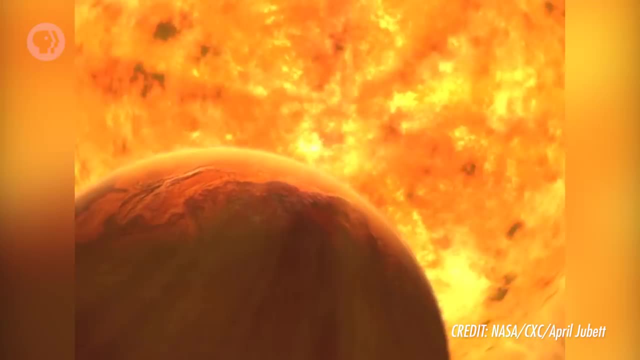 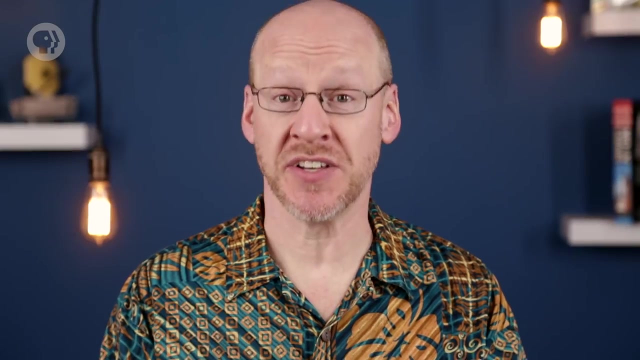 brief, glorious moment. it expands, but then blows away its outer layers, leaving behind the gravitationally compressed core. It goes out with a whimper- Well, a whimper- from a two-octillion-ton, barely-constrained nuclear-powered fireball. 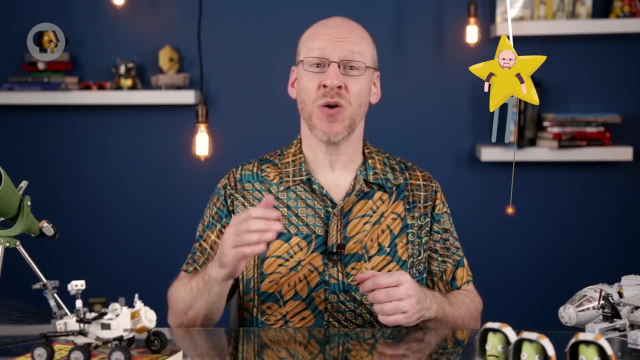 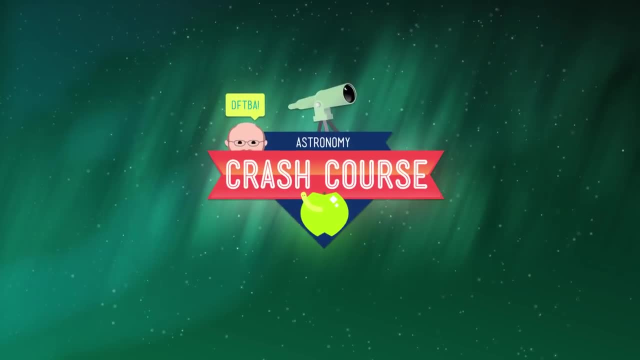 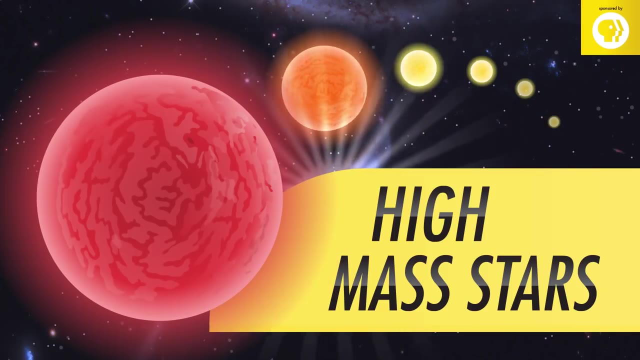 But more massive stars aren't quite as resigned to their fate When they go out, they go out with a bang, A very, very big bang, One giant leap for mankind. In the core of a star, pressure and temperature are high enough that atomic nuclei can get. 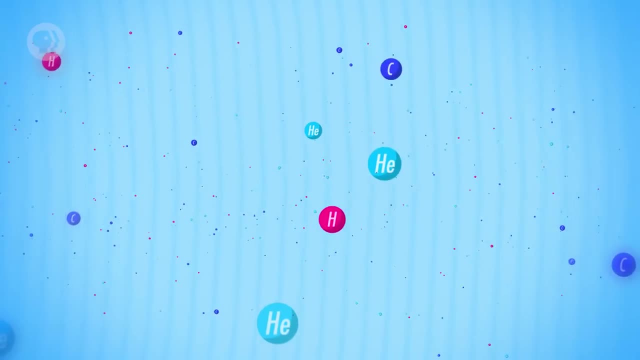 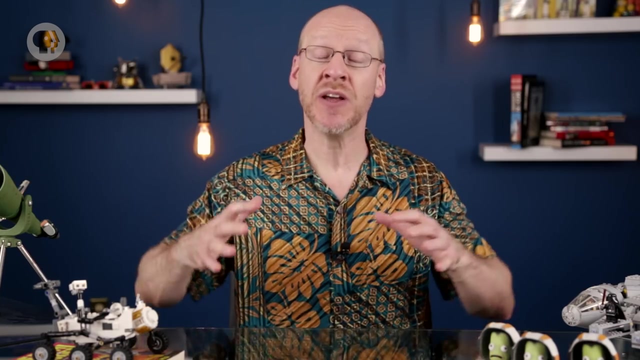 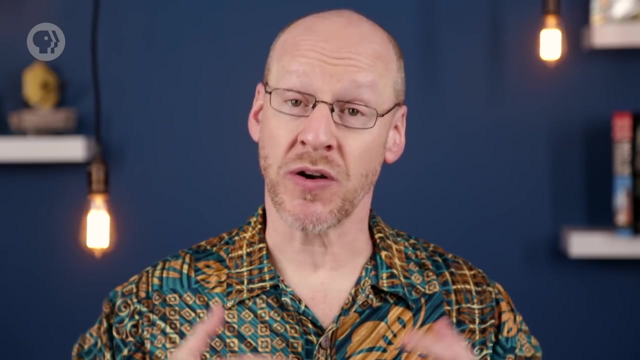 squeezed together And fuse. This releases energy and creates heavier elements. Hydrogen fusion makes helium, Helium fusion makes carbon, And each heavier element in general takes higher temperatures and pressures to fuse. Lower-mass stars like the Sun stop at carbon Once that builds up in the core, the star's. 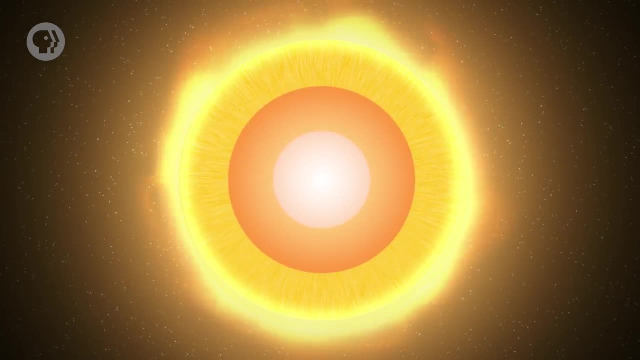 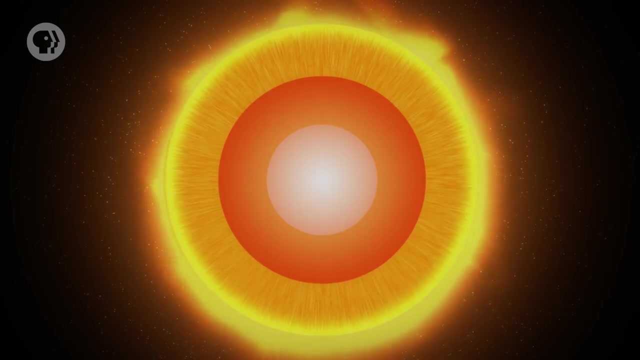 fate is sealed. But if the star has more than about eight times the Sun's mass, it can create temperatures in its core in excess of 500 million degrees Celsius, And then carbon will fuse. There are actually a lot of steps in this process, but in the end you get carbon fusing. 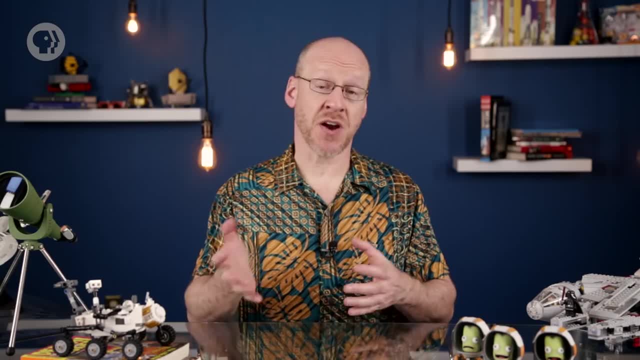 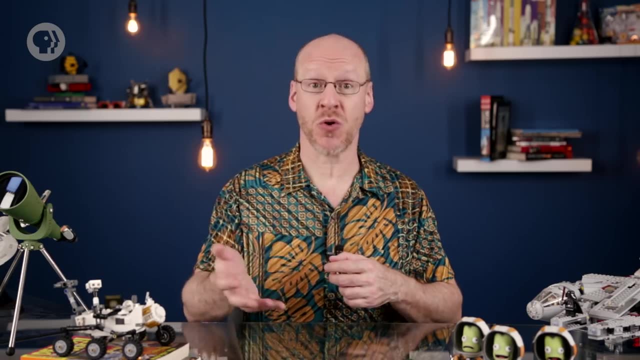 into neon, magnesium and some sodium. What happens next harkens back to what we found goes on in the Sun's core as it ages. Fuse an element, create a heavier one, then that heavier one builds up until the core contracts and heats up enough to start fusing it. 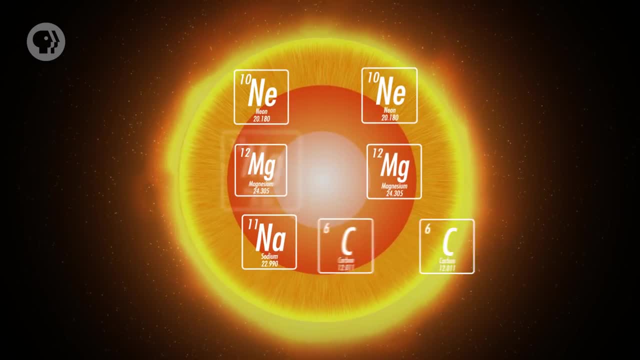 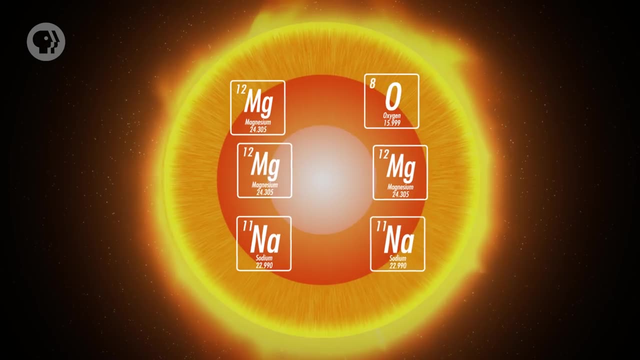 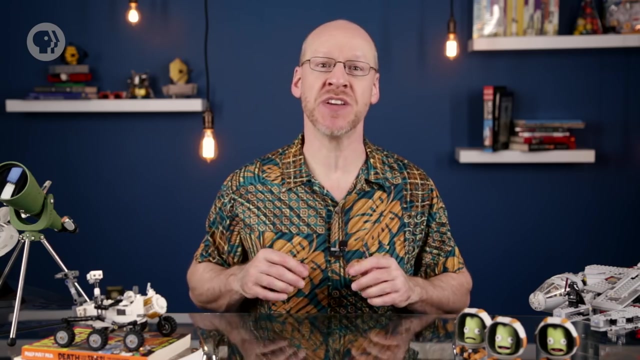 So carbon fusion makes neon, magnesium and sodium, and those accumulate. The core heats up and when it reaches about a billion degrees, neon will fuse. Neon fusion creates more magnesium as well as some oxygen. These build up in the core. it shrinks, heats up to about 1.5 billion degrees and then oxygen fuses, creating silicon. Then that builds up until the temperature hits about 2 to 3 billion degrees, whereupon silicon can fuse Among a pile of other elements. silicon fusion creates iron, And that's trouble, Big, big trouble. Once silicon fusion starts, the star is a ticking time bomb. 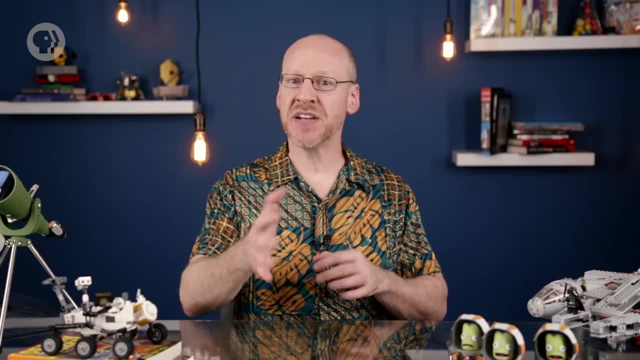 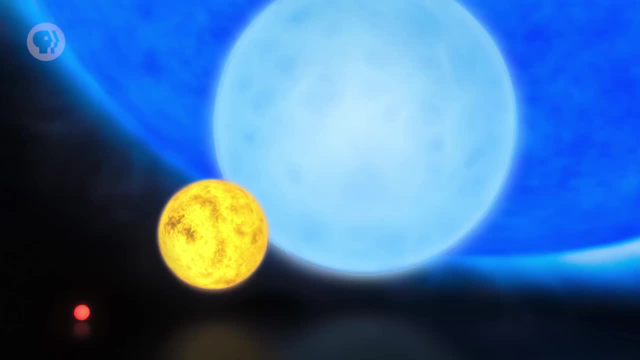 But before we light that fuse, let's take a step back. What's happening to the outer layers of the star? What do we see if we're outside looking back at it? Because the star was born massive. it spent its hydrogen-fusing days as a blue main-sequence. 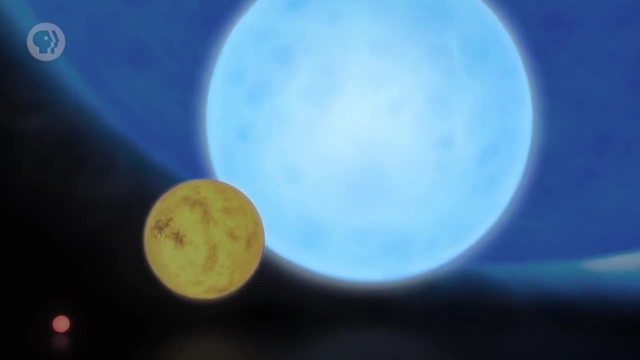 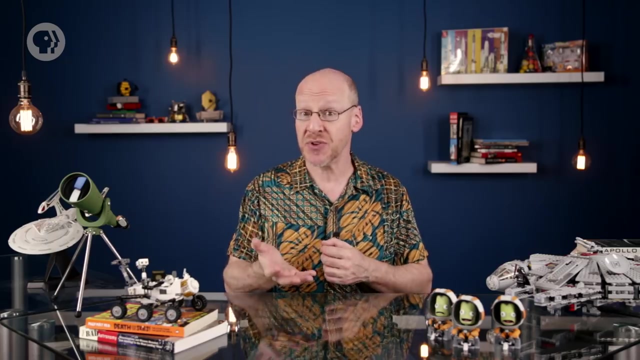 star Stars like this are extremely luminous and can be seen for tremendous distances. Like the Sun, though, a massive star changes. when hydrogen fusion stops, its core contracts and then helium fusion begins. It swells up, just as the Sun will, but instead of becoming 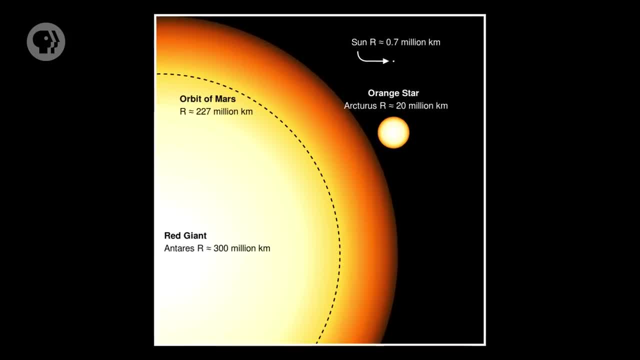 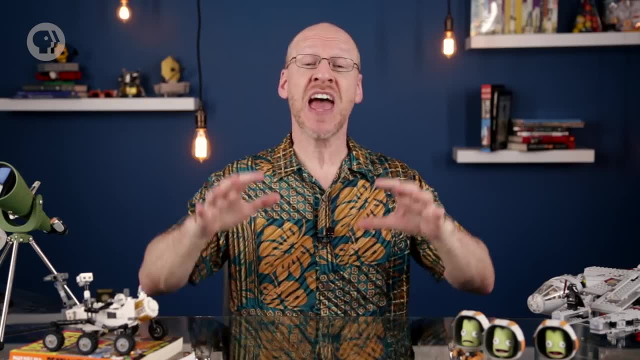 a red giant. it generates so much energy it becomes a red supergiant. These are incredibly huge stars, some over a billion kilometers across, And they are luminous. For example, Betelgeuse in Orion is a red supergiant and one of the brightest. 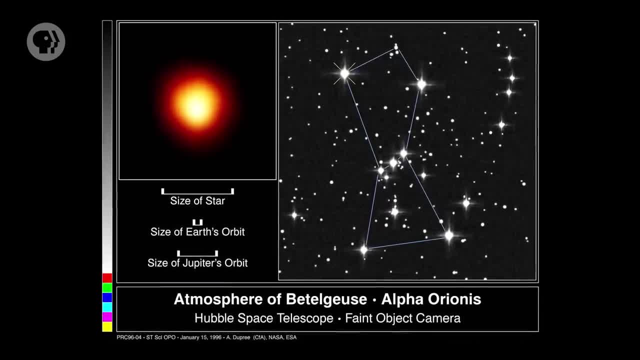 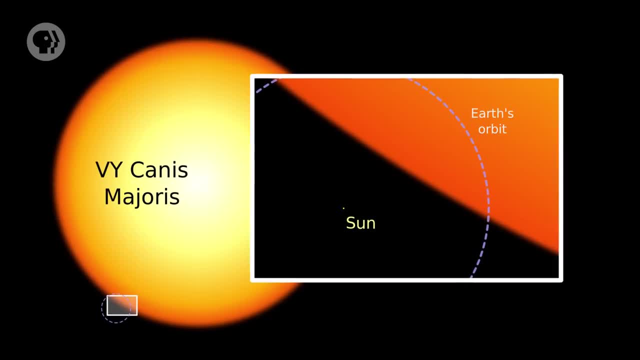 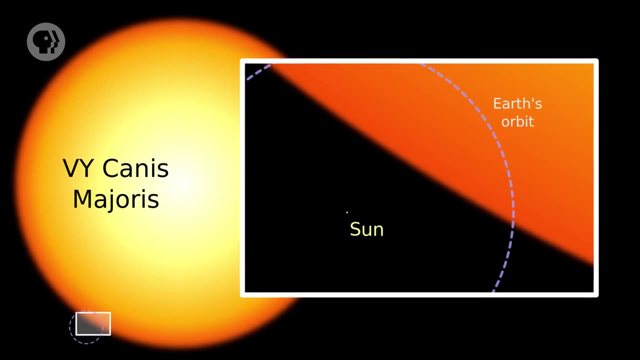 stars in the sky, despite being over 600 light-years away. From that distance, you'd need a decent telescope to see the Sun at all. And that's nothing compared to VY Canis Majoris, the largest known star, which is a staggering 2 billion kilometers across. We even have a special 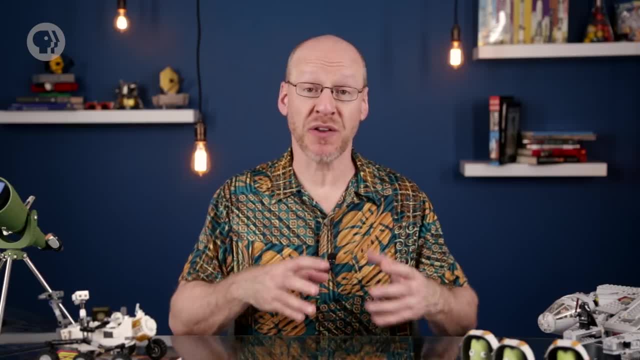 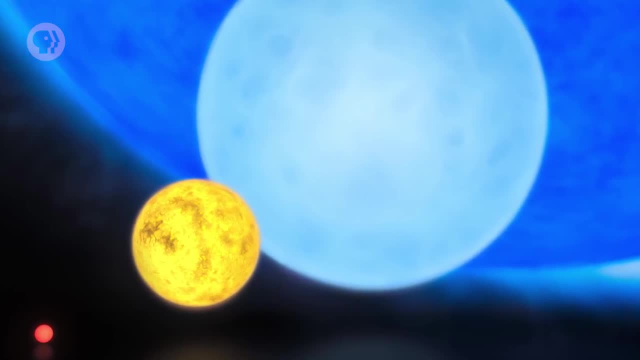 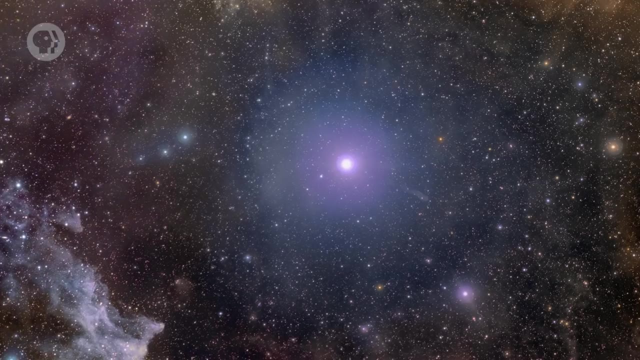 term for it- A hypergiant. As the core switches back and forth from one fusion reaction to the next, the outer layers respond by contracting and expanding. so a red supergiant can shrink and become a blue supergiant. Rigel, another star in Orion, is a blue supergiant putting out over 100,000. 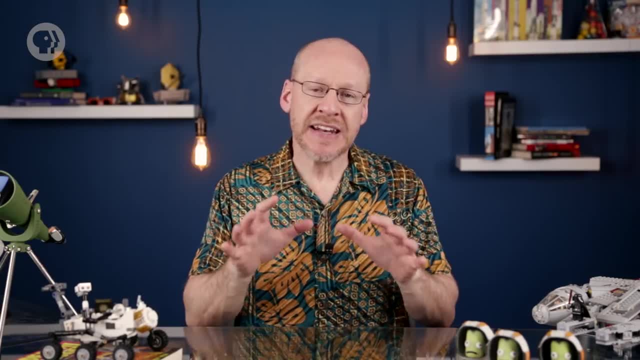 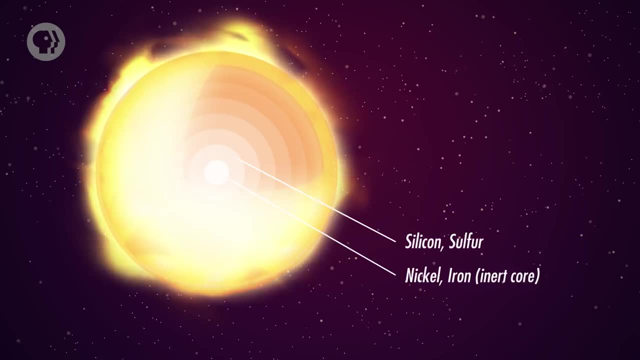 times as much energy as the Sun. OK, let's go back to the core. It now looks like an onion with multiple layers. Iron is building up in the center, surrounded by fusing silicon. Outside that is a layer of fusing oxygen, then neon silver. 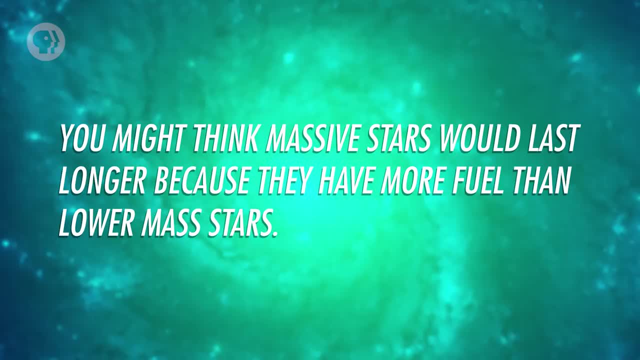 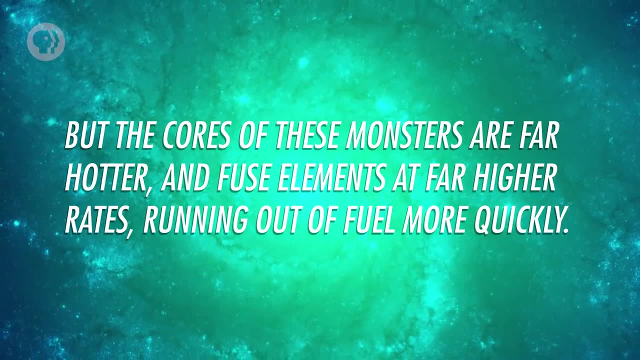 Then neon, then carbon, then helium and finally hydrogen. You might think massive stars would last longer because they have more fuel than lower-mass stars, But the cores of these monsters are far hotter and fuse elements at far higher rates, running out of fuel more quickly. A star like the Sun can happily fuse hydrogen into helium for over 10 billion years, But a star twice as massive as the Sun runs out of hydrogen in just 2 billion years. A star with 8 times the Sun's mass runs out in only 100 million years or so, And each step in the fusion process the sun's mass is 8 times the sun's mass. Each step in the fusion process happens faster than the one before it. In an extreme case, like for a star, 20 times the mass of the Sun. it'll fuse helium for about a million years, carbon for about a thousand, and neon fusion will use up all. its fuel in a single year. Oxygen lasts for only a few months. Silicon fuses at a ridiculously high rate. The star will go through its entire supply in — get this — a day, Yes, one day. The vast majority of a star's mass is just one. day. One star's life is spent fusing hydrogen. The rest happens in the metaphorical blink of an eye. Silicon fuses into a bunch of different elements, including iron. That inert iron builds up in the core just like all those elements did before, And just like before the iron. 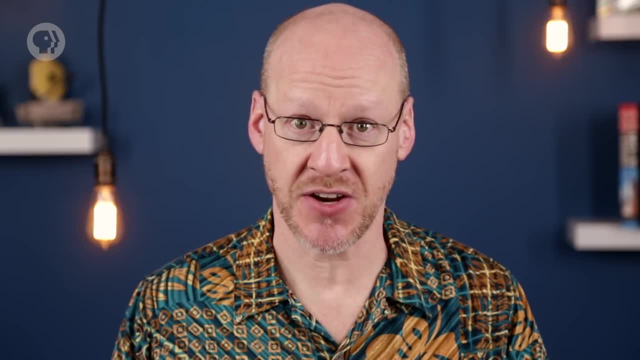 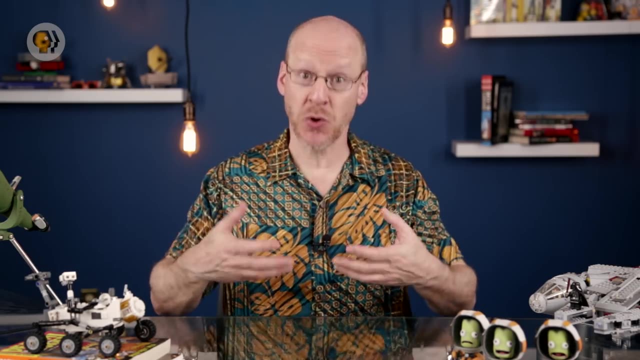 core shrinks and heats up. But there's a huge difference here. In all the previous fusion stages, energy is created, That energy transforms into heat and that helps support the soul-crushing amount of stellar mass above the core. But iron is different. When it fuses it actually sucks in. 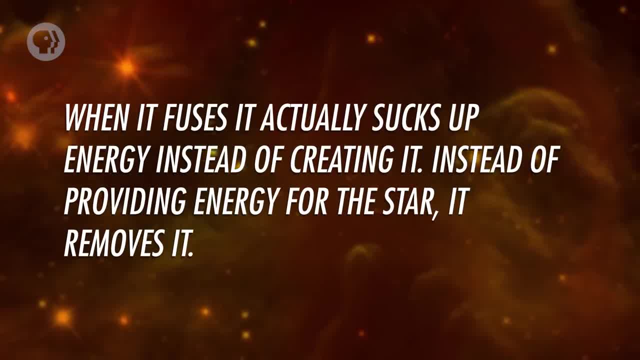 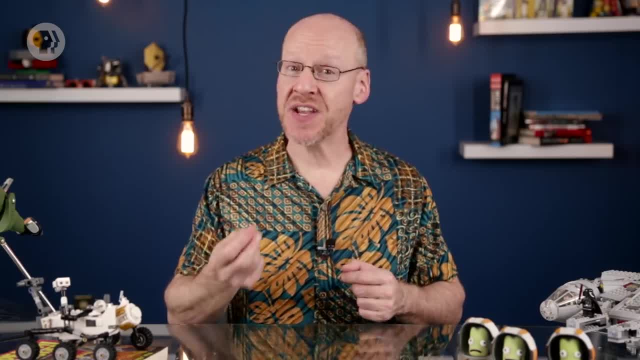 It sucks up energy instead of creating it. Instead of providing energy for the star, it removes it. This accelerates the shrinking, compressing the core, heating it up even more. Even worse, at these temperatures and pressures, the iron nuclei suck up electrons that are whizzing around, which are also helping support the core. It's a double whammy. Both major means of support for the star are removed in an instant. Silicon fusing into iron is happening so fast. this literally takes a fraction of a second once it gets started. The core gets its legs kicked out from under it. It doesn't shrink, it collapses. The gravity of the core is so mind-bogglingly strong that the outer parts crash down on the inner parts at a significant fraction of the speed of light. This slams down on 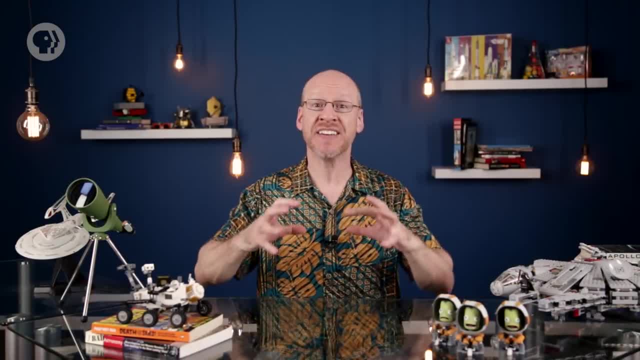 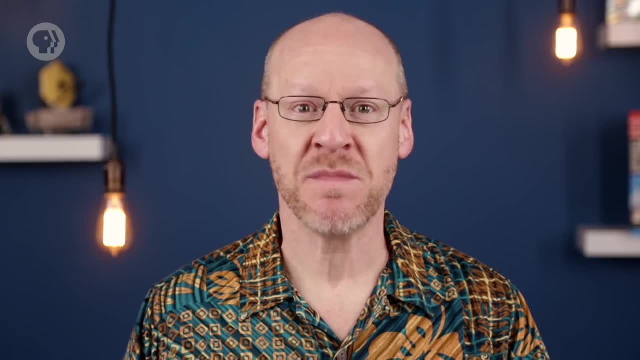 the central core collapsing from several hundred kilometers across down to a couple of dozen kilometers across in just a few thousandths of a second. The star is doomed, because all hell is about to break loose Now. at this point, one of two things can happen. 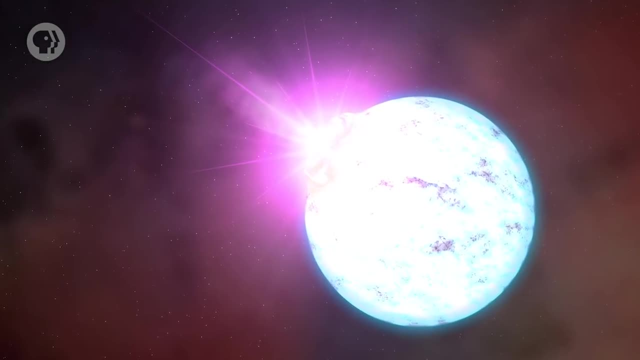 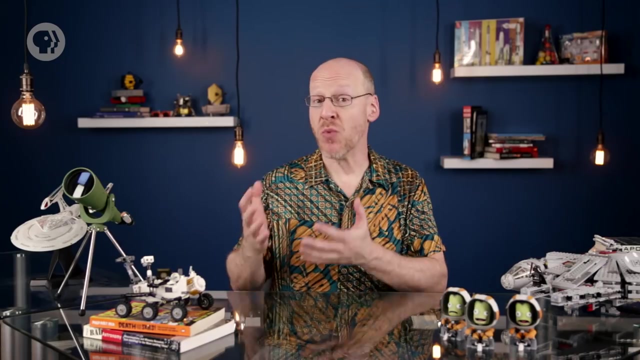 If the star has less than about twenty times the Sun's mass. the core collapse stops. when it's still twenty or so kilometers wide, It forms what's called a neutron star, which I'll cover in the next episode. If the star is more massive than this, then the collapse cannot be stopped by any force. 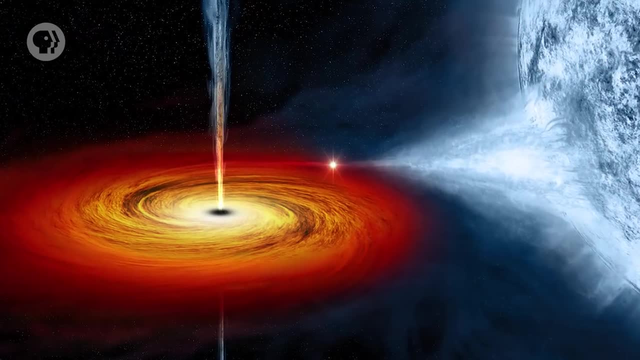 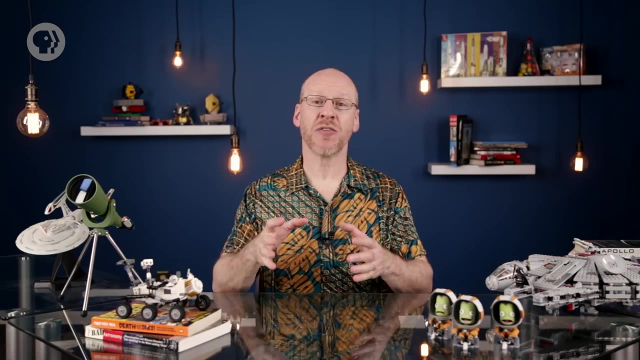 in the Universe. The core collapses all the way down down to a point. The gravity becomes so intense that not even light can escape. A black hole is born. We'll cover black holes in a future episode as well, But for now, what happens when the 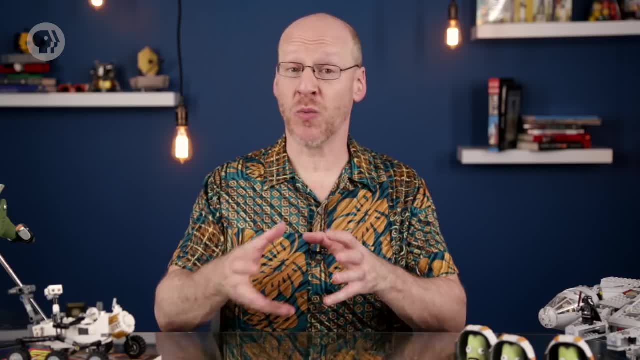 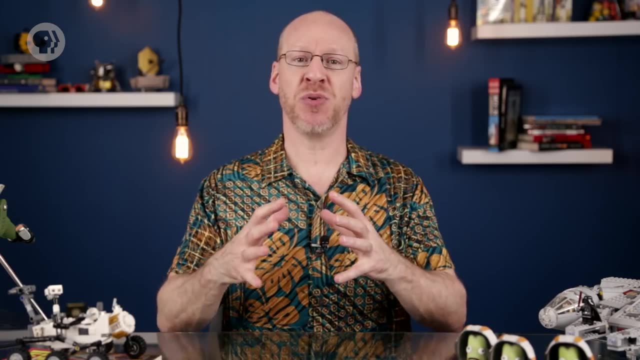 core collapses. It collapses and suddenly stops. The core of the star, whether it's a neutron star or a black hole, is now extremely small. with terrifyingly strong gravity. It pulls on the star's matter above it hard. This stuff comes crashing down at a fantastic speed and gets hugely compressed, ferociously heating up. At the same time, two things happen in the core. While this stuff is falling in, a monster shockwave created by the collapse of the core moves outward and slams into the incoming material. The loss of energy is so insane it slows down that material substantially. 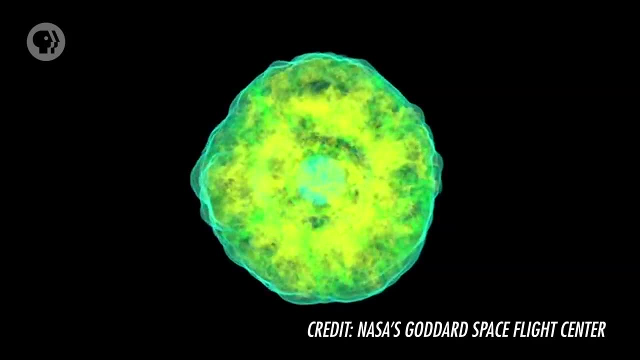 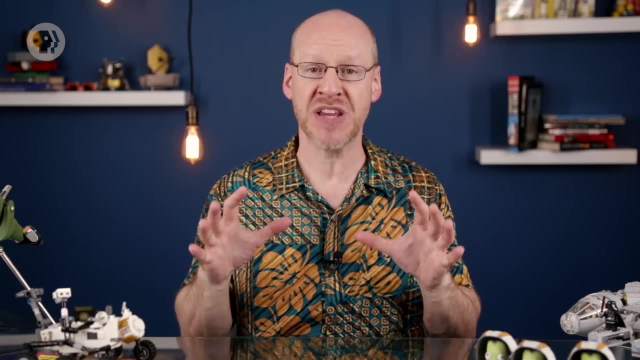 The second event is that the complicated quantum physics brewing in the core generates vast numbers of subatomic particles called neutrinos. The total energy carried by these little neutrinos is almost beyond reason. In a fraction of a second they carry away 100 times as much. 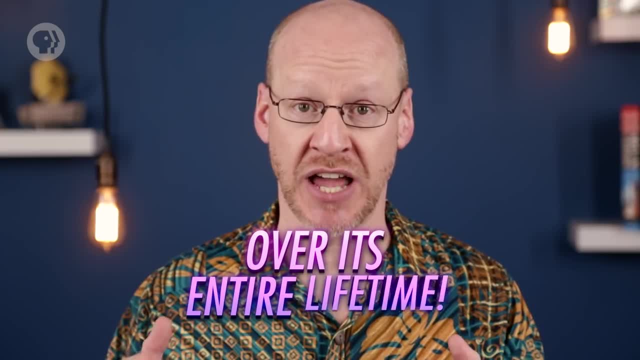 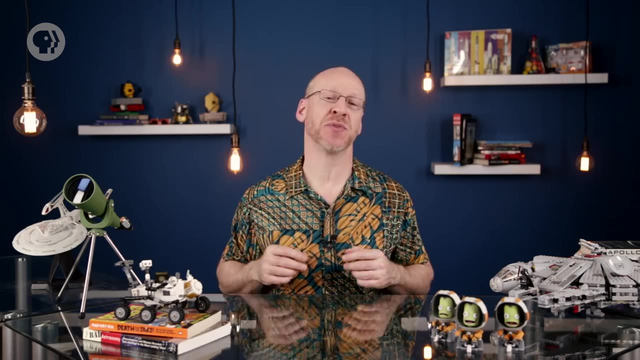 energy as the Sun will produce over its entire lifetime. That's an incredible amount of energy. Now, these little beasties are seriously elusive and hate to interact with normal matter. One single neutrino could pass through trillions of kilometers of lead without even noticing. 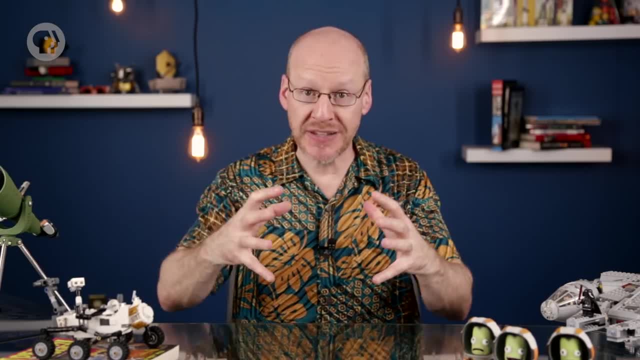 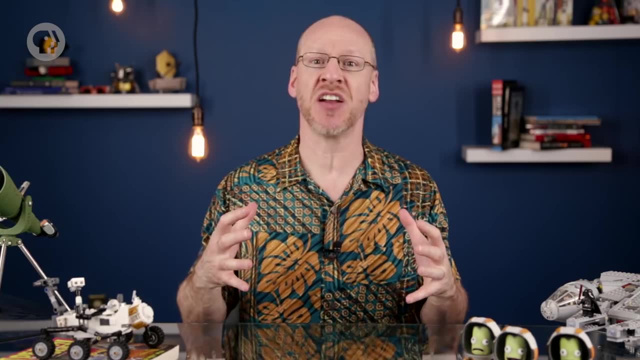 But so many are created in the core collapse and the material barreling down on the core is so dense that a huge number of them are absorbed. This vast wave of neutrinos slams into the oncoming material like a bullet train hitting a slice of warm butter. The material, 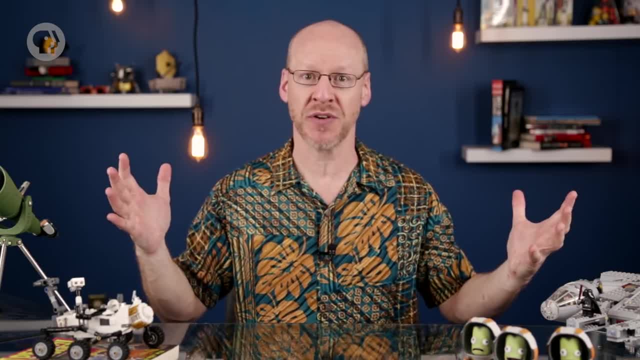 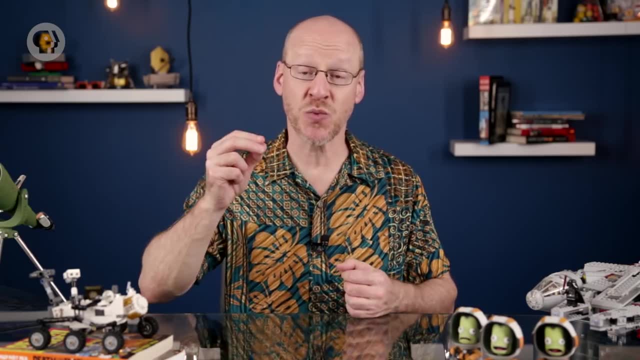 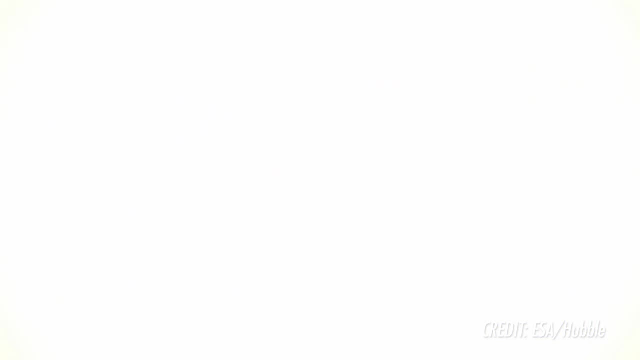 stops its infall, reverses course and blasts outward, The star explodes. It explodes, Poof. This is called a supernova and it is one of the most violent and terrifying events the universe can offer. An entire star tears itself to shreds and the expanding gas blasts. 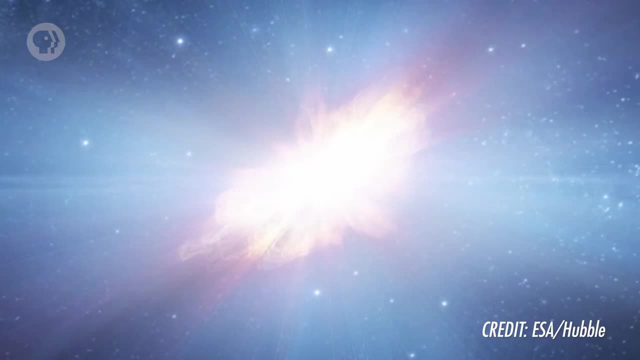 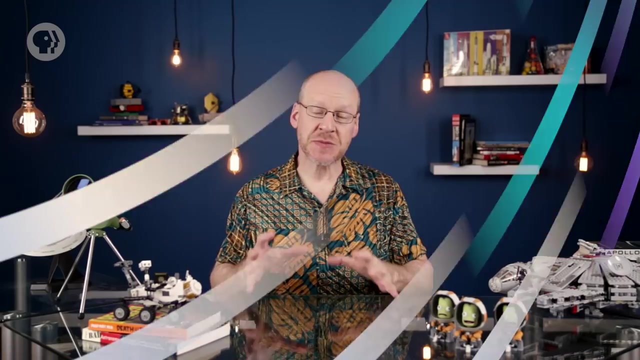 outward at 10% the speed of light. The energy released is so huge they can be seen literally halfway across the universe. They outshine all the stars in the rest of the galaxy combined. The expanding material called the supernova remnant forms fantastic shapes, The most. 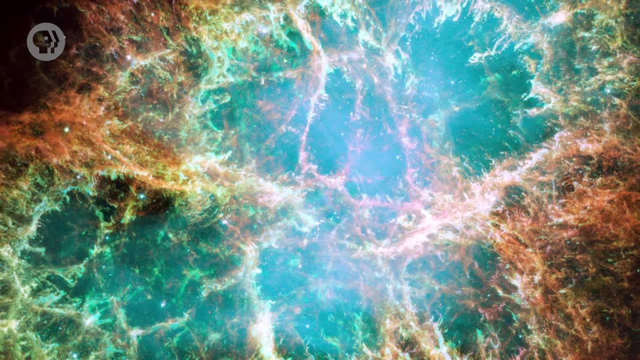 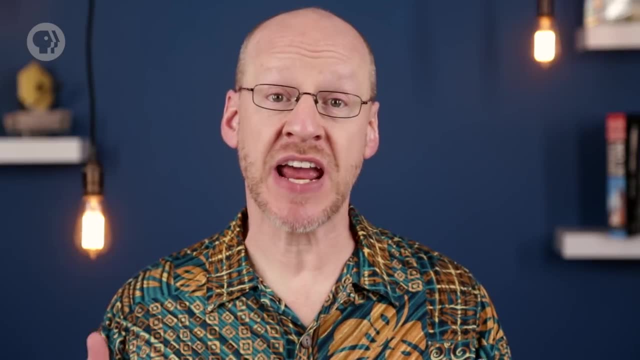 famous is the Crab Nebula from a star we saw blow up in the year 1054. The tendril as the material expands into the gas and dust that surrounded the progenitor star. As remnants expand and age, they become more tenuous. Some have bright rims as they push. 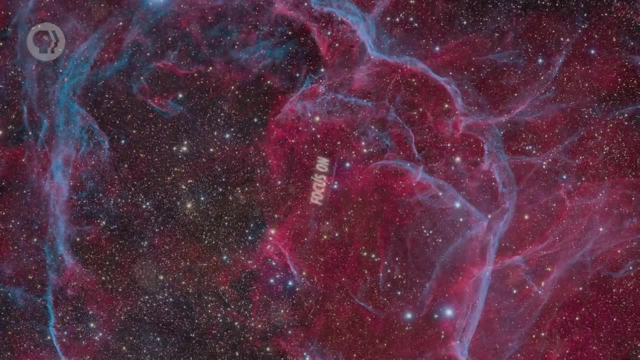 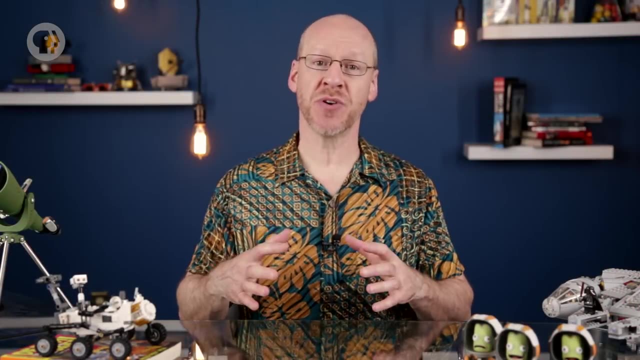 into material between the stars. Others form complex webs of filaments. I'm often asked if there are any stars near enough to hurt us when they explode. The quick answer is no. Even though supernovae are incredibly violent, space is big. A supernova would have. to be at least as close as 100 light-years from us before we start feeling any real effects. The nearest star that needs to explode is the Crab Nebula. from a star we saw blow up at 10% the speed of light. The Crab Nebula. from a star we saw blow up at 10% the speed. of light. The nearest star that needs to explode is the Crab Nebula. from a star we saw blow up at 10% the speed of light. The nearest star that needs to explode is the Crab Nebula. from a star we saw blow up at 10% the speed of light- The nearest star that needs to. 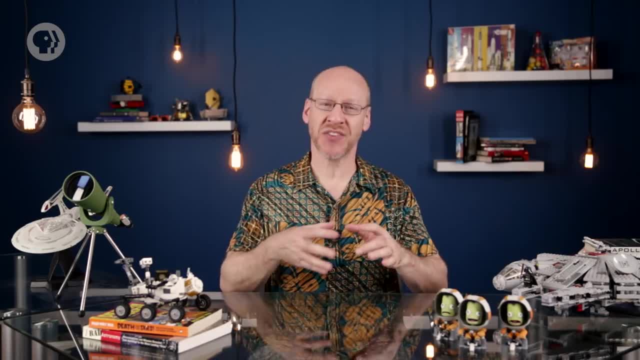 explode is the Crab Nebula, from a star we saw blow up at 10% the speed of light. The nearest star that might explode in this way is Spica, in Virgo, and it's well over 100 light-years away. I say might explode because it's at the lower mass limit for going supernova — it. 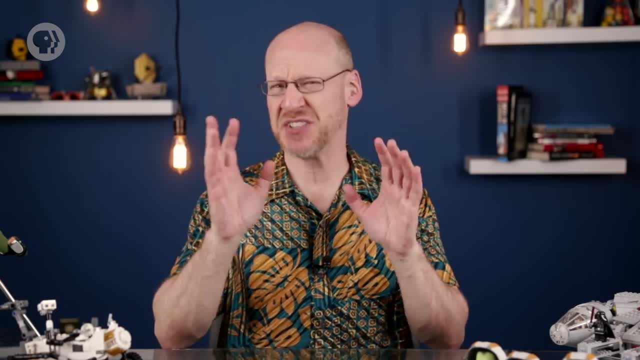 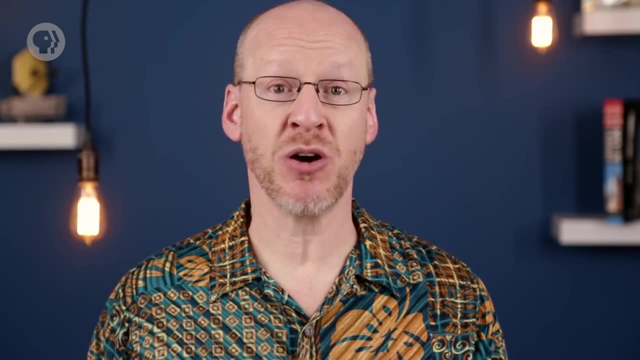 might not explode at all. Beetlejuice will certainly explode someday, but it's too far away to hurt us. We're pretty safe from this particular threat. I'll note that after all this, there is another kind of supernova involving white dwarfs, which we'll cover in our episode about binary stars. Happily, we're probably. 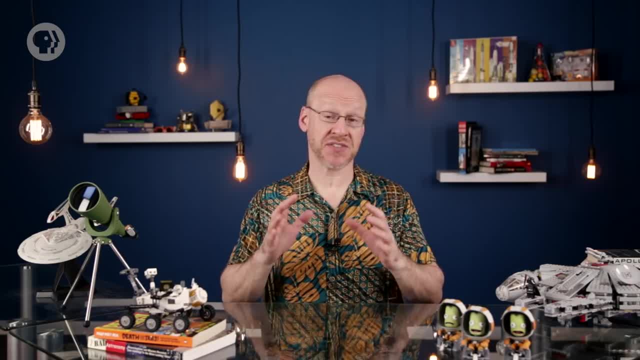 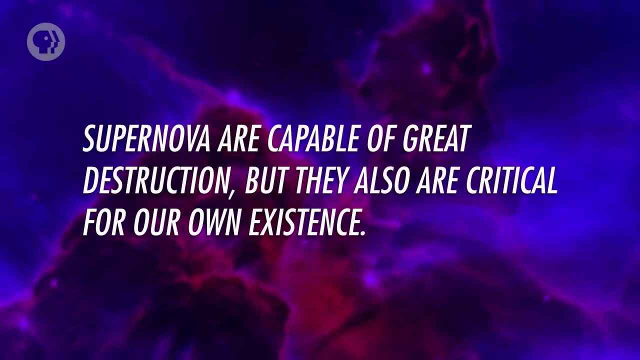 safe from them too, Breathe easy. As terrifying and dangerous as supernovae are, there's a very important aspect of them you need to know. Supernovae are capable of great destruction, but they're also critical for our own existence. When the star explodes, the gas gets so hot and is compressed so violently. 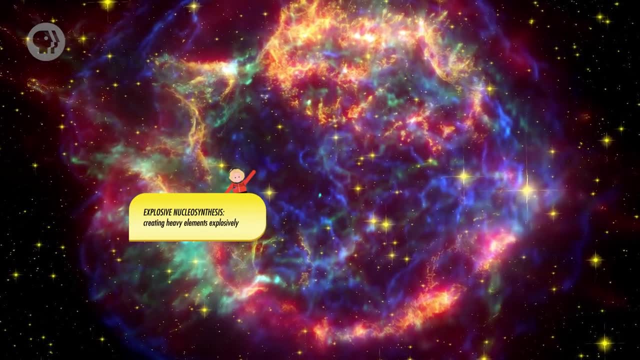 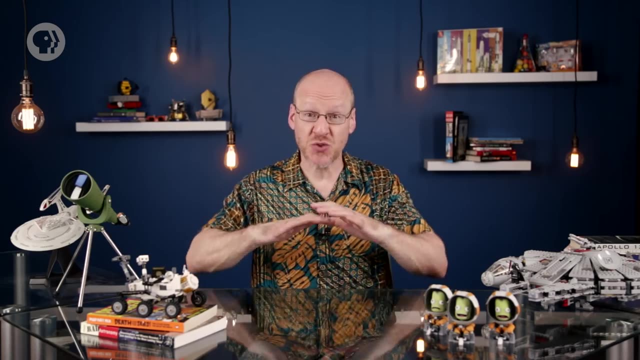 by the blast that it undergoes, fusion, what astronomers call explosive nucleosynthesis, literally creating heavy elements. explosively, New elements are produced in quantities that dwarf the Earth's mass: Calcium, phosphorus, nickel, more iron, all made in the hellish. 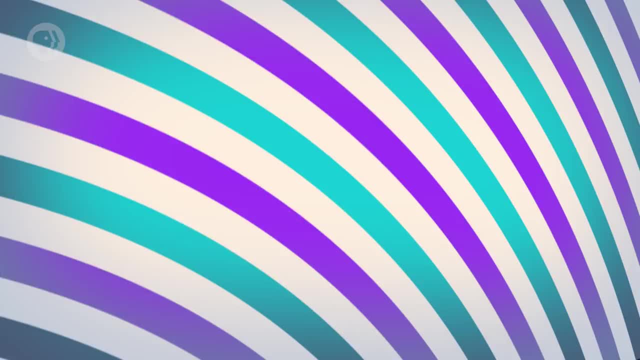 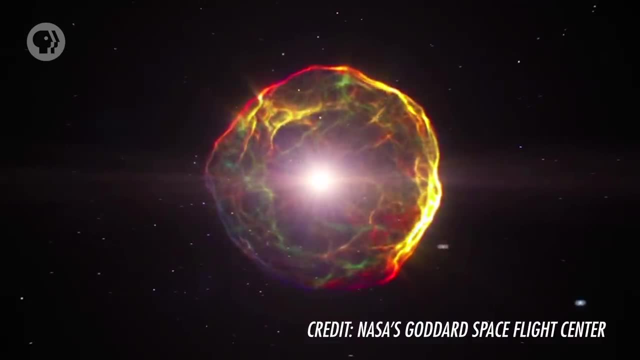 forge of the supernova heat and flung outward into the universe. It takes millennia or longer, but this material mixes with the other gas and dust clouds floating in space. Sometimes these clouds will be actively forming stars, Sometimes the collapse of the cloud to form. 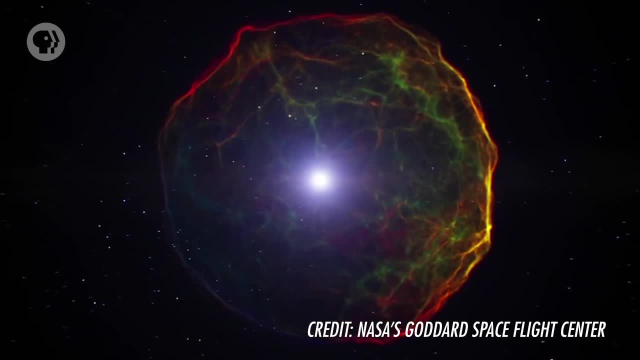 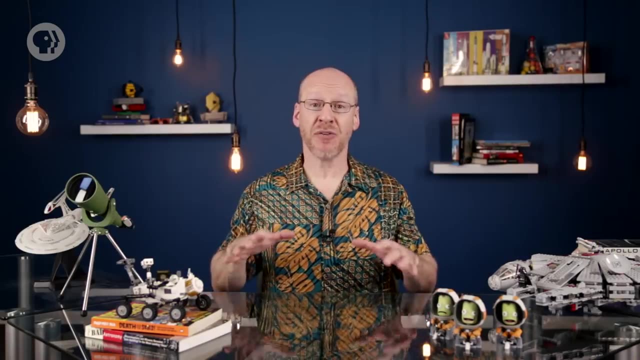 stars may even be triggered by the supernova slamming into it. Either way, the heavy elements created in the supernovae are capable of destroying the universe. Supernovae will become part of the next generation of stars and planets. Supernovae are how the 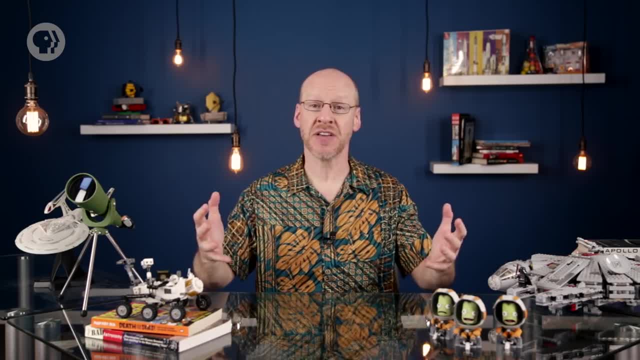 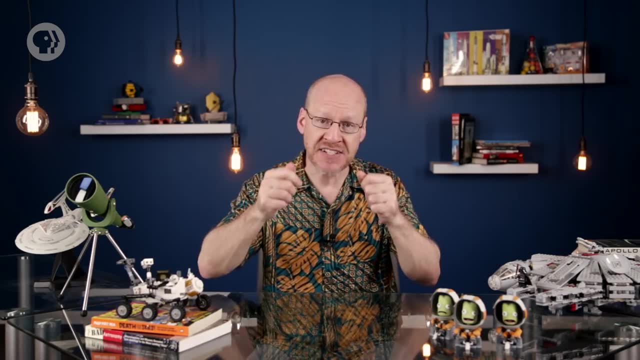 majority of heavy elements in the universe are created and scattered: The calcium in your bones, the iron in your blood, the phosphorus in your DNA — all created in the heart of the titanic death of a star. That star blew up more than 5 billion years ago, but parts of it go on — in you. Today, you learned that massive stars fuse heavier elements in their cores than lower-mass stars. This leads to the creation of heavier elements up to iron. Iron robs critical energy from the core, causing it to collapse. The shock wave. 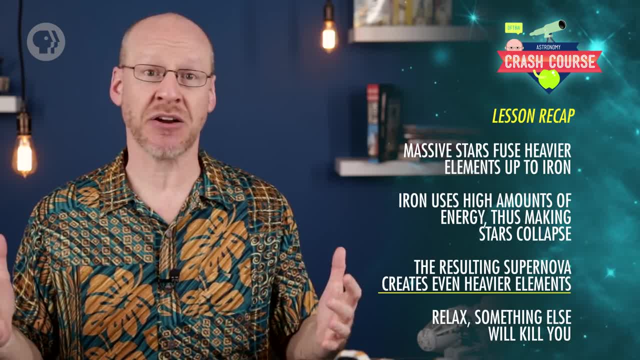 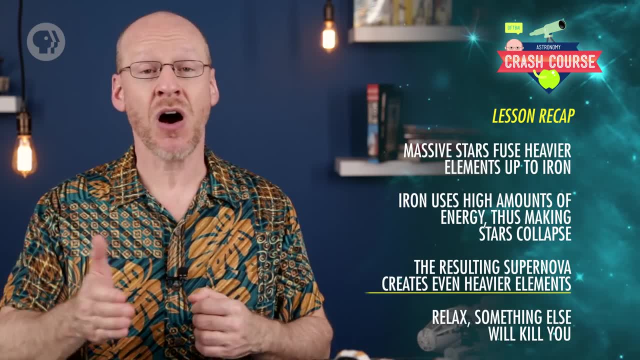 together with a huge swarm of neutrinos, blasts through the star's outer layers, causing it to explode. The resulting supernova creates even more heavy elements, scattering them through space. Also, happily, we're in no danger from a nearby supernova. 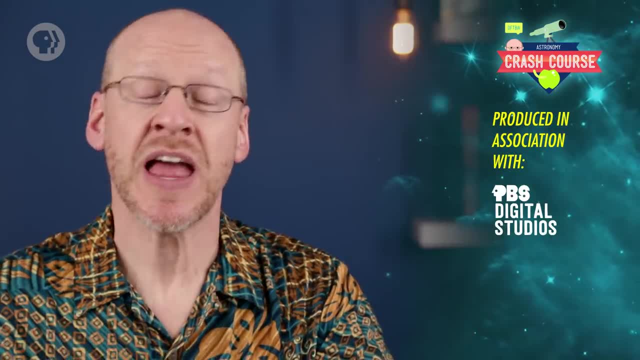 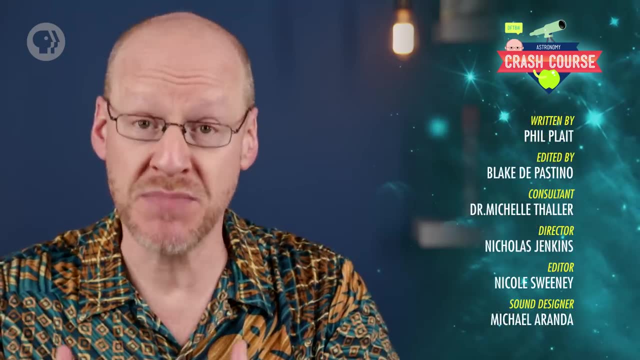 Crash Course Astronomy is produced in association with PBS Digital Studios. They have a YouTube channel with great videos. Go, just go over there, check their videos out. They're fantastic. The script was edited by Blake T Pastino and our consultant is Dr Michelle Thaller. 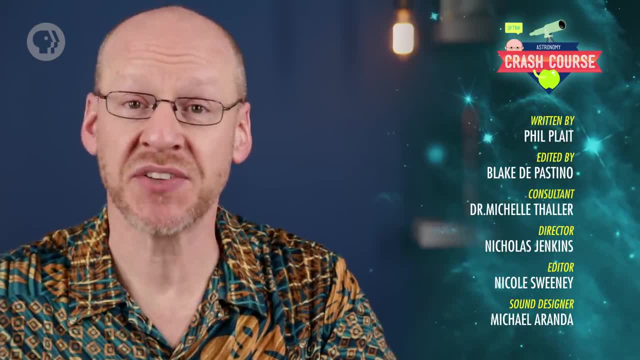 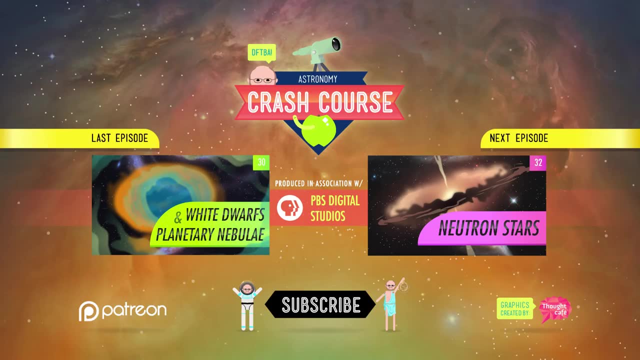 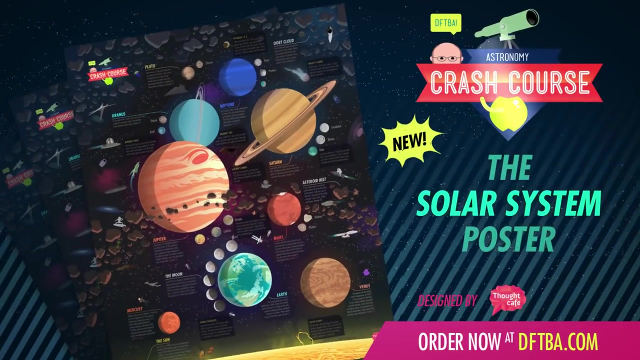 It was directed by Nicholas Jenkins, edited by Nicole Sweeney, The sound designer is Michael Aranda and the graphics team, as always, is Thought Cafe, Subtitles by the Amaraorg community.